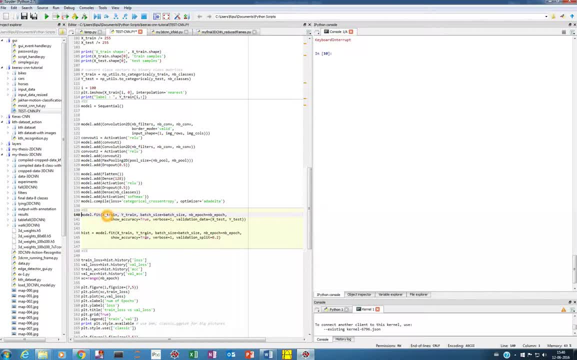 there, if you remember. Only what is to do is we just do model fit and we start training this, But in order to visualize it, we will assign a variable to it, A hist variable, which means history, and this hist variable will store all the 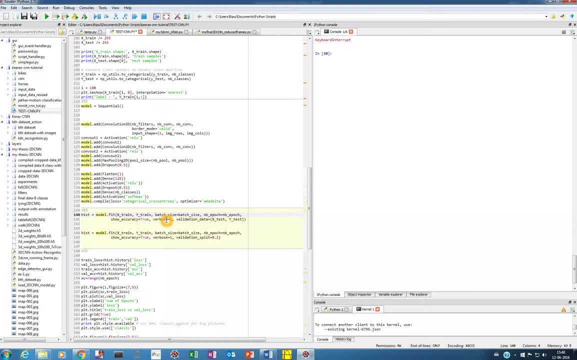 loss and accuracies during training, of both validation as well as the training data. So from there we can plot the graphs and all. So let me run this command. So it will take some time. So I will pause the video and I will get back to you when the time comes. 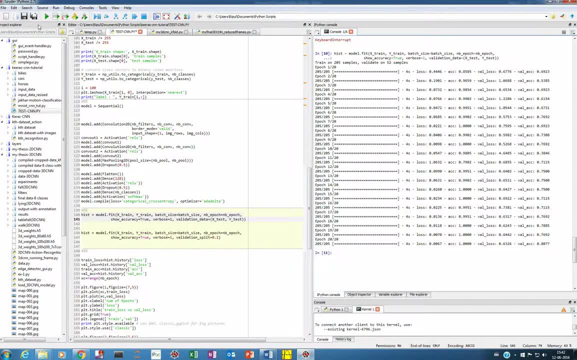 Training is complete. So once my training is complete, as you can see, while training we have four variables. One is loss and accuracy. This refers to training loss, training accuracy and this is the validation loss and the validation accuracy. So in my case, I have manually splitted. 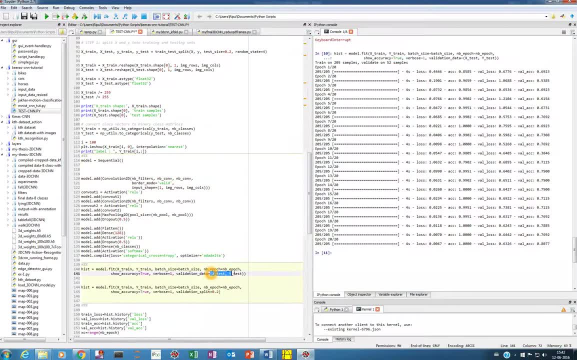 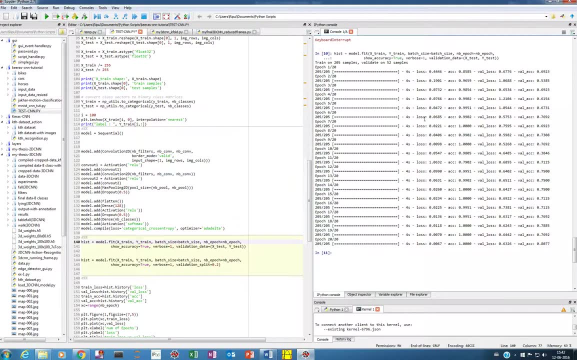 the data into training and test, and the test data I was using as a validation. If you don't want to do it manually, you can use this command. And so now, how we can visualize this, how the things are changing as per the number of epochs. 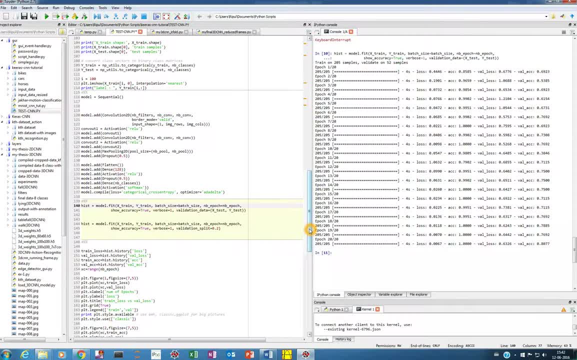 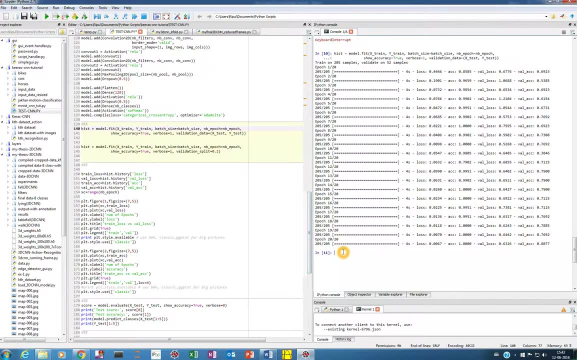 Here there are very less epochs- 20. But people when they are training big networks, they have more than 1000 epochs or something. So what you do is we have four variables and you can see here. if you see the hist, just type here hist and ok. ok, I think hist. 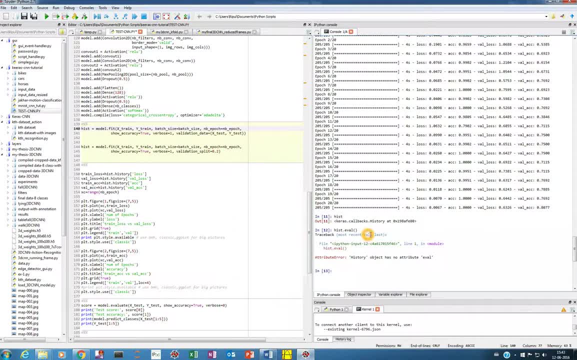 Ok, maybe this is not the command I don't remember. Ok, so we will visualize it later. Now let's see this first. So now what I will do is I will give a name training loss as histhistoryofloss. Ok, I think this should be the command. I forgot it: Histhistory. 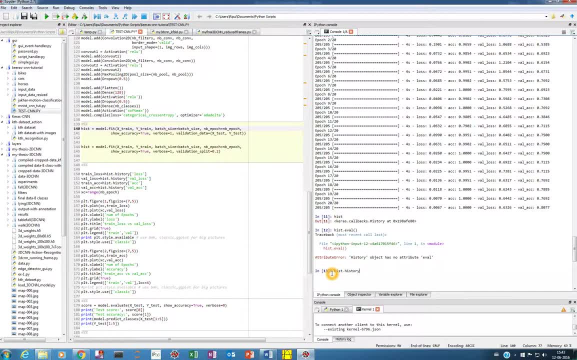 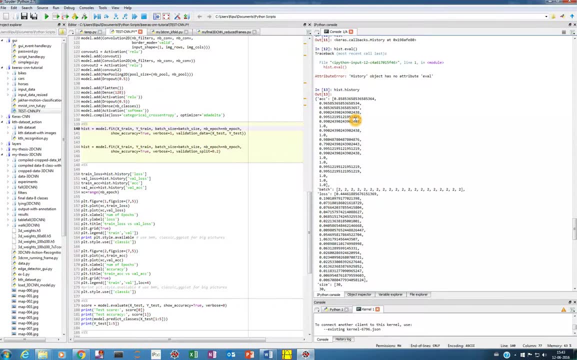 Let's see if it works out. Yeah, so here is the command So you can see Histhistory. So it's showing you the accuracy, The 20 accuracy, First epoch, second epoch, and all This is the training accuracy. Then it's showing the batch size which we took two. Then it's. 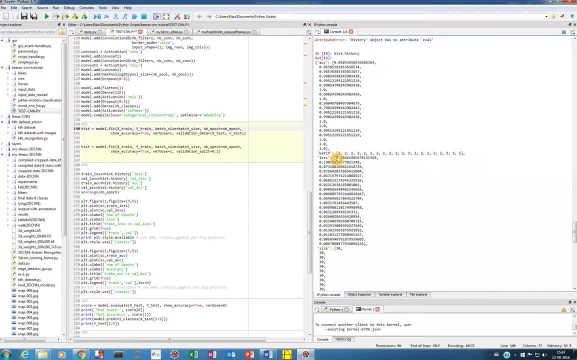 showing the loss- Ok, 20 losses- of each epoch. There will be 20 such losses. And then there is a validation accuracy And validation loss. You can see it, Ok, So there are four or six variables, I guess, Of which we are interested in. 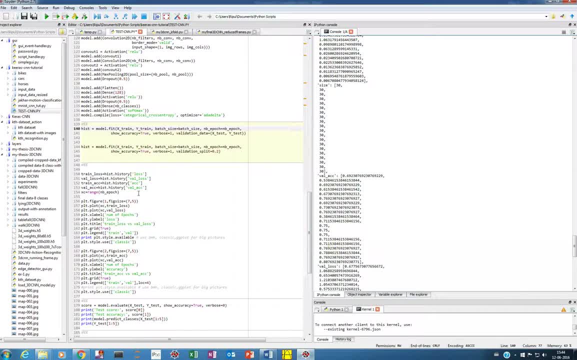 Accuracy loss, validation accuracy and validation loss. So you will use this command From the histhistory. we will take the loss For validation loss. we will take the validation loss For training accuracy. we will take accuracy For validation accuracy. we will take this And. 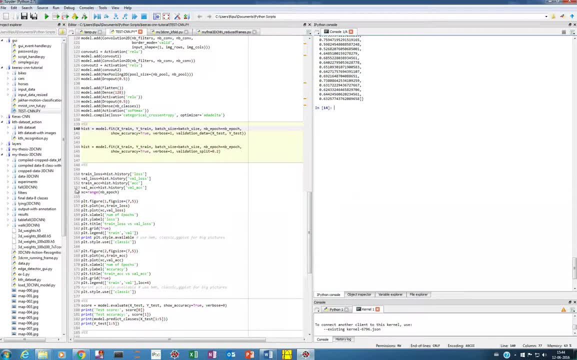 the range which we will give is number of epoch. Ok, And this is simply a plotting. This code is for plotting this graph And you can get this code in my blog. I will give you the link below. So let me run this first So you can see here. This is the training loss versus validation. 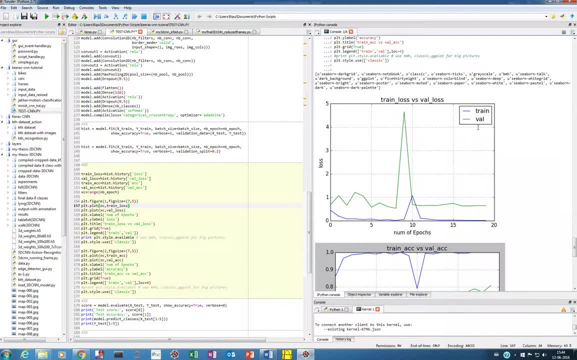 loss. This blue color is the training loss And this green color, I guess, is the validation loss. So from here you can see how the training loss is decreasing. Then there is a P. Actually this is not a robust network, So you cannot see the graphs going very nicely, Like the. 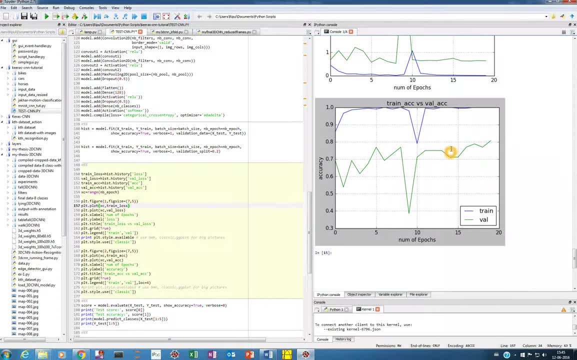 curves, shape going down, And same is the accuracy. So, as per your network, I mean, you can visualize it and you can then change the parameters in order to get a better graph in which the system is learning. So that's all for this video. Use this code and you can visualize your graph for training, loss and even the